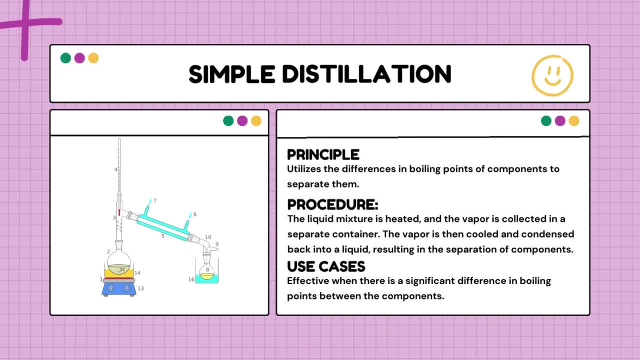 get started with the simple distillation. firstly, talking about simple distillation, simple distillation is a method of separating the components in a liquid mixture based on the differences in their boiling point. the mixture is heated and the component with the lowest boiling point vaporizes first. the vapor is then condensed back into a liquid in a separate container, and that results. 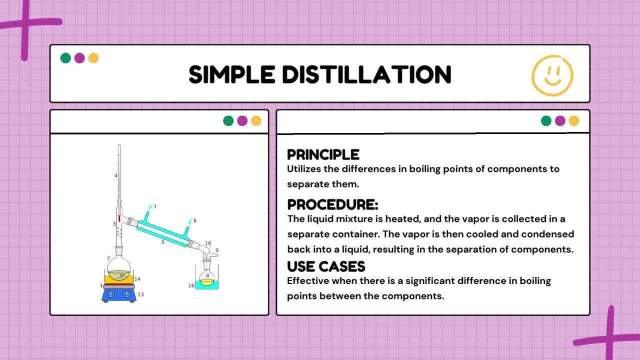 in the isolation of the individual components. this process is effective when there are significant differences in boiling points and among the components. okay, so this was a brief about simple distillation. now we'll be looking at the principle of simple distillation. so simple distillation relies on the fact that different substances 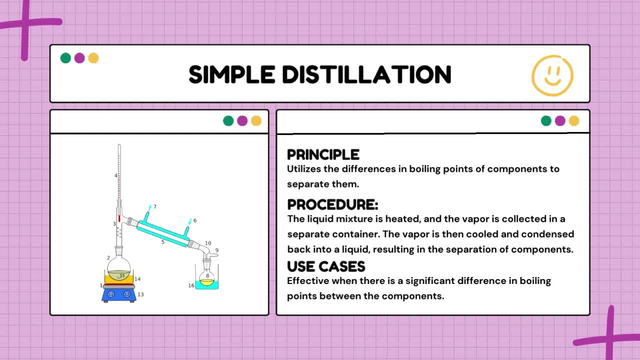 in a mixture have different boiling points and by exploiting these differences you can separate the component effectively. to understand this clearly, imagine that you have a mixture of liquids and they each have their own temperatures at which they like to become gas. simple distillation uses these preferences to separate them. now looking at the 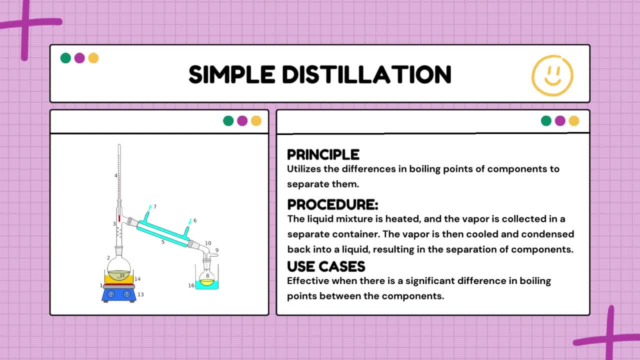 procedure. it all starts with the heating stage. the liquid mixture is gently heated. this is a start to give the mixture a bit of thermal energy. as the mixture is heated, the component with the lowest boiling point starts turns into vapor. now, in this separate container, the vapor is cooled down. the cooling process is crucial because it 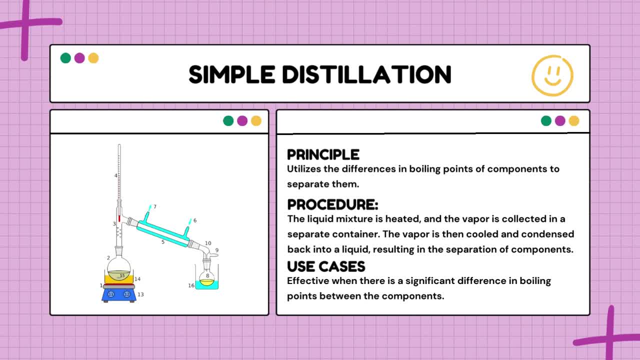 transforms the vapor back into a liquid. the cooling and condensation results in the isolation of the individual components. since each component has its unique boiling point, they transforms back into the liquid at different temperatures. this temperature based transformation is what enables the separation. so, guys, this was the procedure of simple distillation. 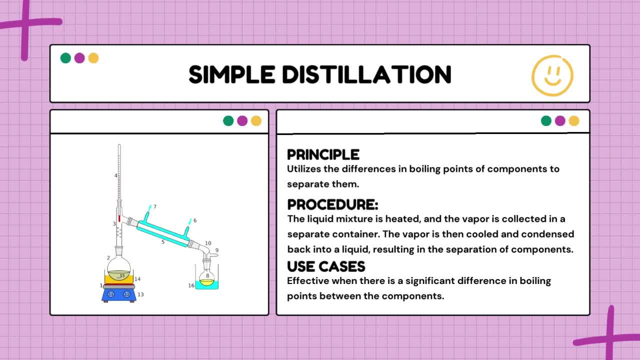 now we'll look at where is simple distillation used. simple distillation gives extraordinary results when they are subjected to difference in boiling point among the components. if the components which are mixed together has a large difference in their boiling points, simple distillation becomes a reliable method for separating the components into individual components. so, guys, this was a brief. 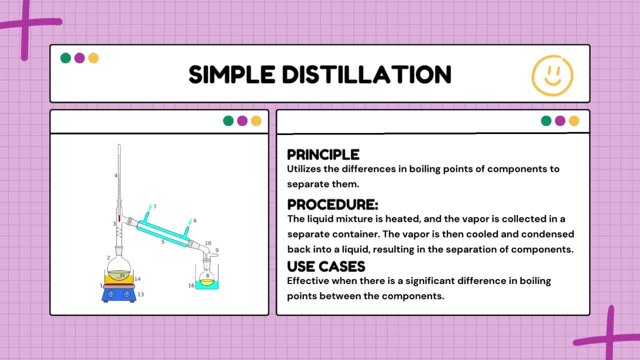 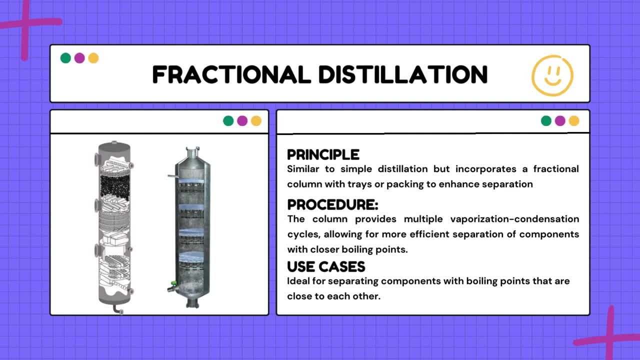 about simple distillation. now we'll be looking at the next type of distillation, which is fractional distillation. fractional distillation is a technique used to isolate different components in a liquid based on the distinct boiling points. it builds upon the principle of simple distillation, but adds a specific column to enhance the precision. talking about its principle, we need to just imagine fractional distillation. we need to imagine the fractional distillation as a bigger and advanced version of simple distillation. however, the fractional column adds a layer of complexity and precision to the routine. 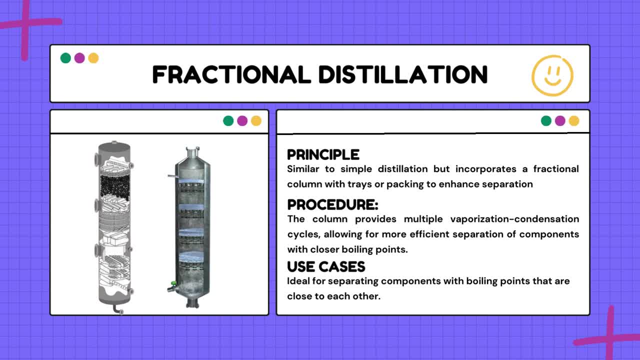 looking at the procedure of fractional distillation, it all starts with the heating stage. similar to simple distillation, you start by gentle heating the liquid mixture after heating stage. next is about the fractional column. the fractional column is the main magic where everything starts. here the vapor rises through the fractional column, which is through the trays or packing materials. these surfaces provides opportunity for the vapor to condense and re-evaporate the vapor. 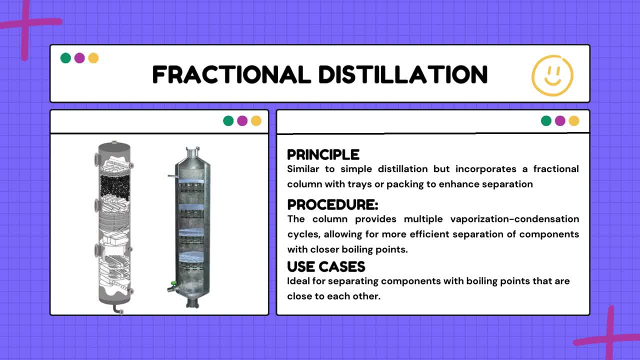 multiple times, enhancing the purity of the products. these repeated cycles of condensation and vaporization in the column creates different temperature zones, and this allows the component with boiling points that are close to each other to have more chances to separate. okay, and this is how the separation of liquids takes place in the fractionation column. and, guys, fractional distillation takes the stage when you are dealing with a liquid mixture, where the components have a 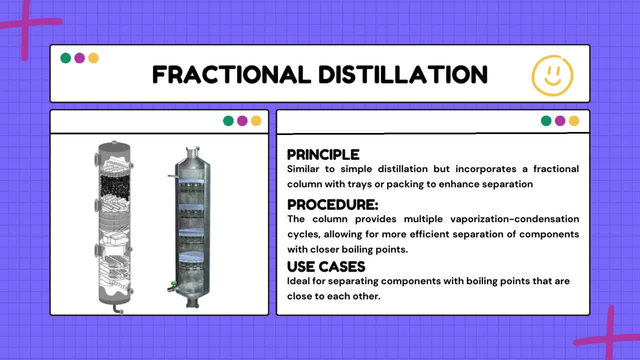 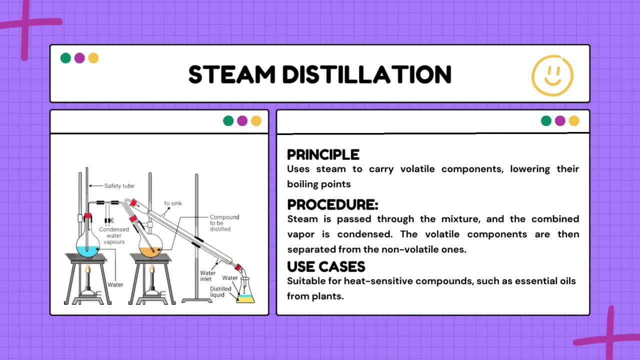 boiling point that are closer to one another on the temperature spectrum. okay, so, guys, this was about a brief of fractional distillation. now we will be looking at the next type of distillation, which is steam distillation. guys, steam distillation is a method that uses steam to elevate volatile components from a mixture. at lower temperatures, it is ideal for extracting the delicate substances, like essential oil, from the plants. 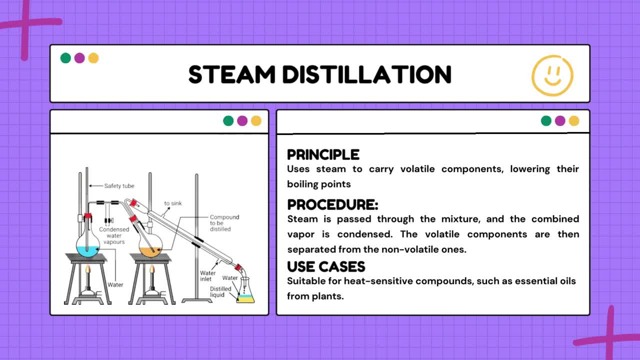 without subjecting them to high temperature. the principle is like as an elevator for volatile components in a mixture. it's like giving them a lift and making them escape more easily by lowering their usual boiling points. to understand the procedure of steam distillation, imagine that you have a mixture and the components are bit shy about turning into vapor. steam distillation is like the friendly neighbor that encourages them. steam is passed through the mixture and the Pewter types, which are dependent upon the steam nation. 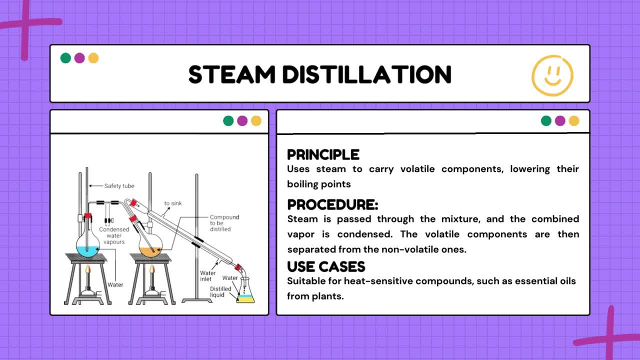 and it acts as a partner, making them feel comfortable in turning them to vapor. The mixture and the steam gets steam-upped and creates a combined vapor. The combined vapor contains both the steam and the now vaporized volatile components, But this journey can't last forever and the combined vapor is condensed. 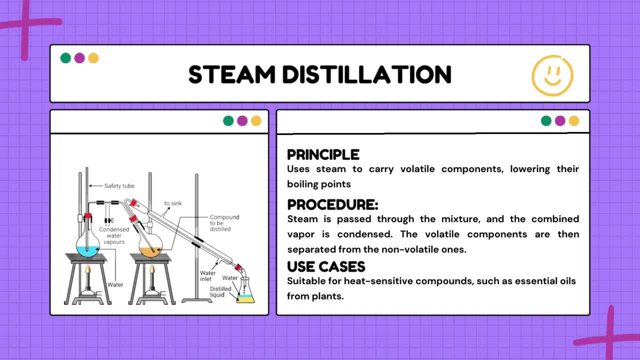 This now turns it back into a liquid. But now you have a mix of water and the volatile components, and the final act involves the separation of volatile component from the water. Since it is not difficult for water to turn back into liquid, it's easier to separate from more elusive volatile components. 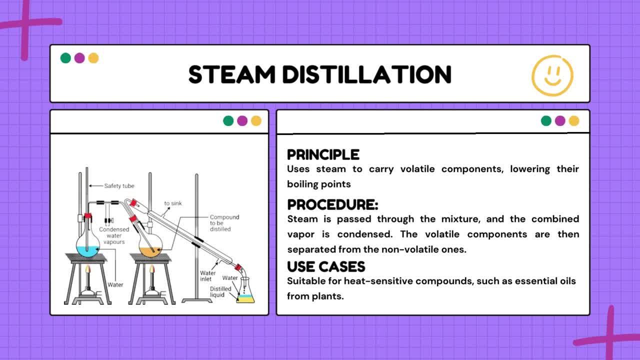 And guys at the end, steam distillation is like a superhero for heat sensitive components. It's like when you are dealing with delicate substances like essential oil in the plants which can get damaged by high temperature, Steam distillation is the go-to method. 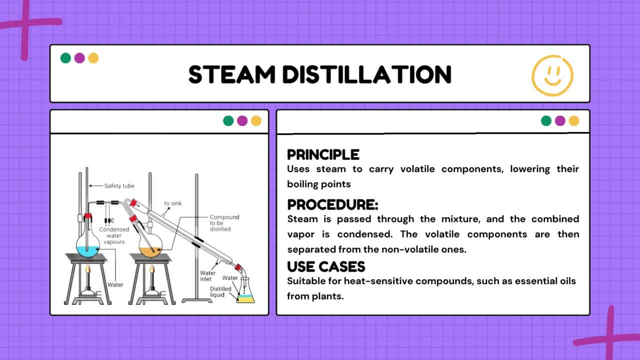 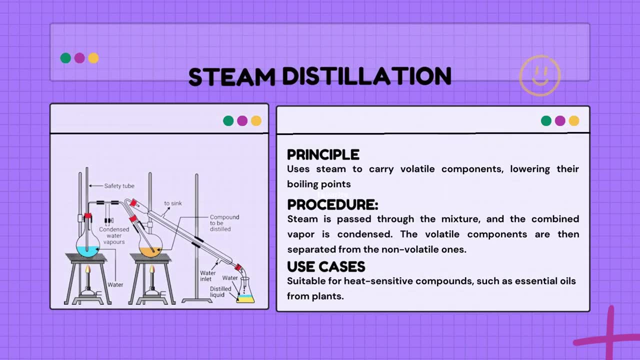 It's a gentle process That ensures the component can get extracted without losing their essence due to excessive heat. Okay, guys, so this was about steam distillation. Now, guys, we will be looking at the next type of distillation, which is vacuum distillation. 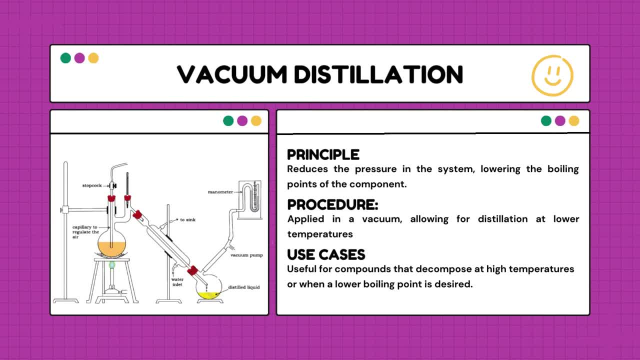 Guys, vacuum distillation is a method that distills the components in a mixture at lower temperature by reducing their pressure, making it ideal for sensitive substances And also where a lower boiling point is desired. Guys, to understand the principle of vacuum distillation, think of the vacuum distillation. 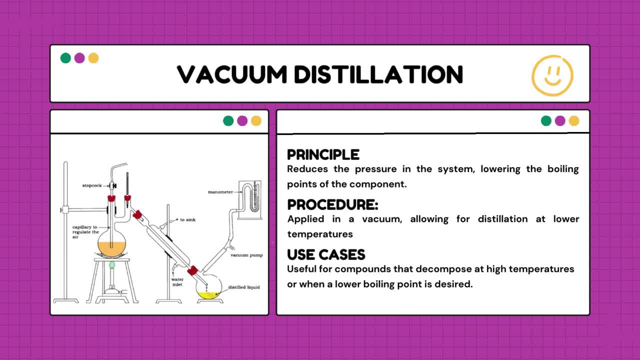 as giving the mixture a makeover by changing the atmospheric pressure rules, By lowering the pressure in the system. it's like telling the components: you can start turning into a vapor at much cooler temperatures. I hope the principle is clear to you. Now looking at the procedure, 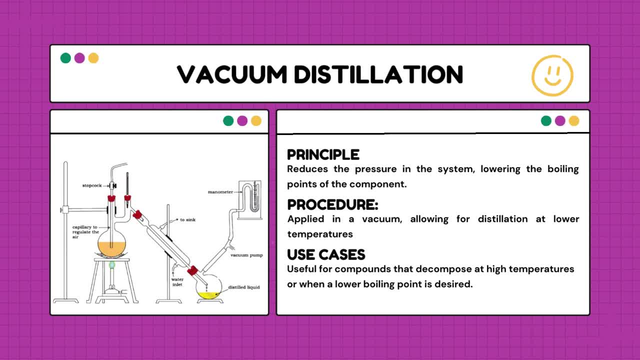 Instead of distilling under the regular atmospheric pressure, vacuum distillation happens in a vacuum where the pressure is intentionally reduced. This change in pressure lowers the boiling point of the components in the mixture And with the drop in the pressure the components start transforming into a vapor at lower temperatures. 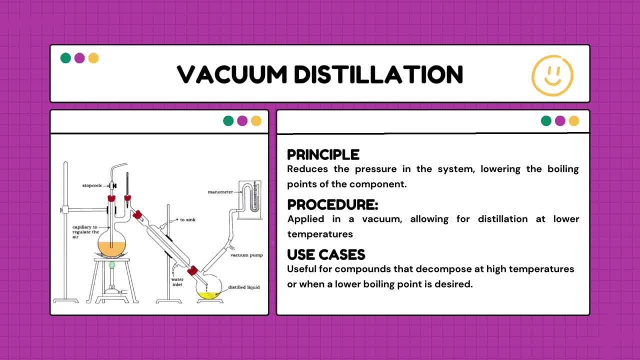 than they would under normal conditions. This reduced temperature means a gentler distillation process, And this is especially handy for distillation. So let's get started. For the components that might get grumpy and break down at high temperatures- And guys talking about the uses- vacuum distillation comes to rescue when you are dealing with. 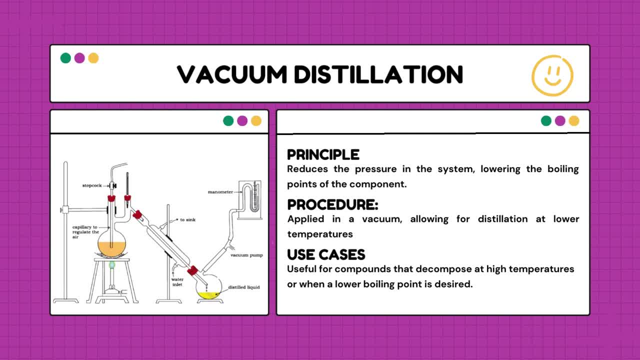 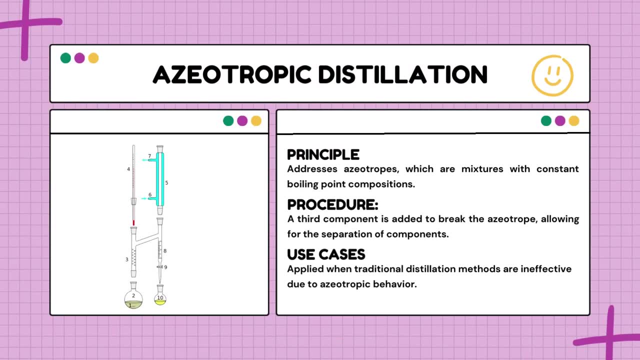 the components that cannot handle the heat, or while dealing with the components which needs excessive amount of heat to break down. I hope this type of distillation is clear to you. Now, moving on with the next type of distillation, that is, azotropic distillation. 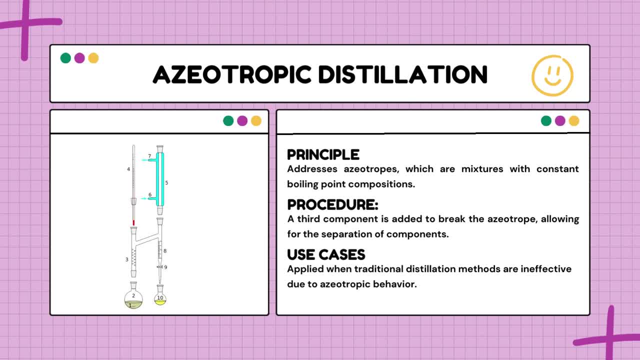 Guys, azotropic distillation is a method for separating mixtures with constant boiling point by introducing a third component to disrupt their behavior and making the separation possible. Now, looking at the principle of azotropic distillation: Azotropes are tricky because they maintain a constant boiling point and making them difficult. 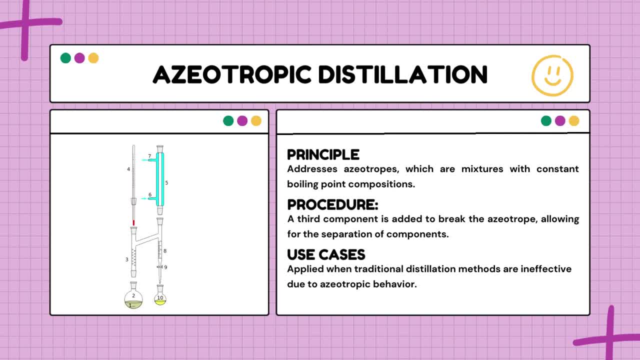 to separate using traditional method. The principle here is to introduce a third component to disrupt their behavior and making the separation possible. So let's get started. So let's start with the first component that disrupts this azotropic behavior or that breaks this azotropic behavior. 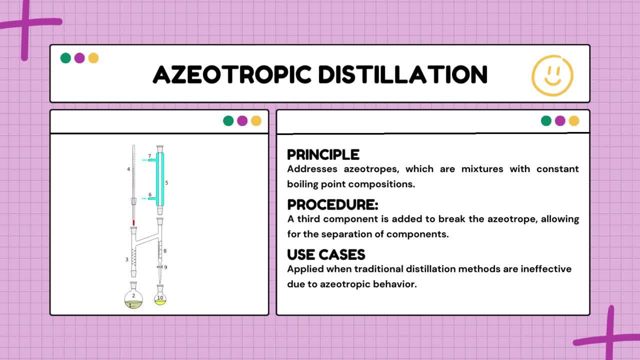 Now looking at the procedure. In azotropic distillation a third component is introduced. This third component breaks the constant boiling point composition of the azotrope. The added component changes the dynamic, breaking the azotropic behavior And with the azotrope disrupted. traditional distillation method can now be applied more. 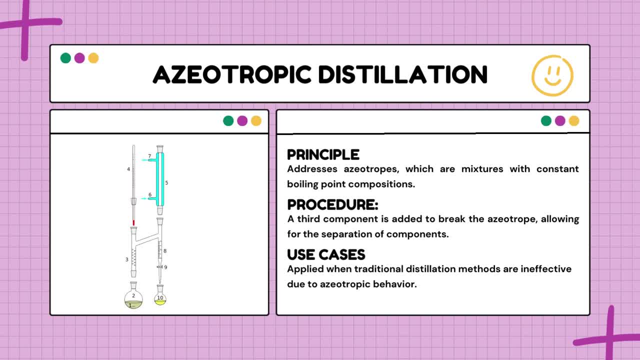 effectively. These components now can be separated into, each following its own distinct boiling points. So, guys, this was the procedure about azotropic distillation. Now talking about the use cases. Azotropic distillation steps in when the traditional distillation method throws their hand up in. 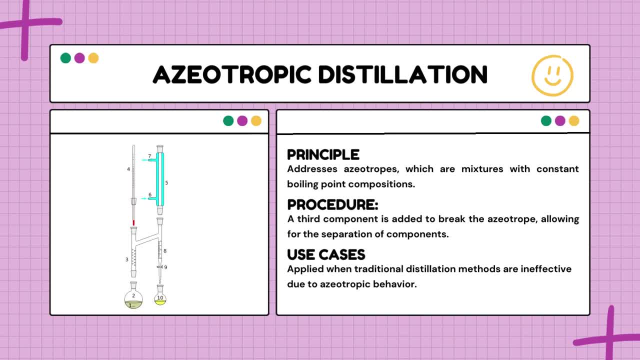 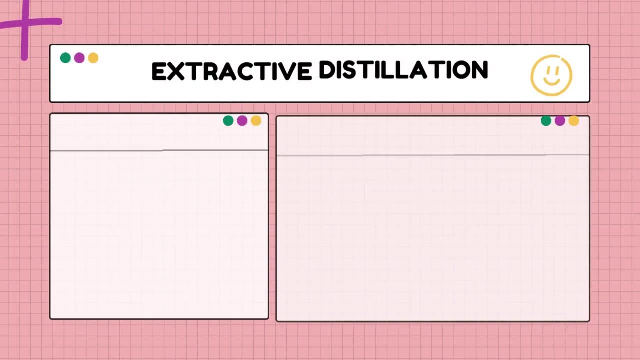 a defeat due to azotropic behavior. If you have a mixture that just won't separate because of the constant boiling point, azotropic distillation won't. It becomes the problem solver. So, guys, this was about the azotropic distillation. Now, lastly, we would be discussing the last type of distillation, which is extractive distillation. 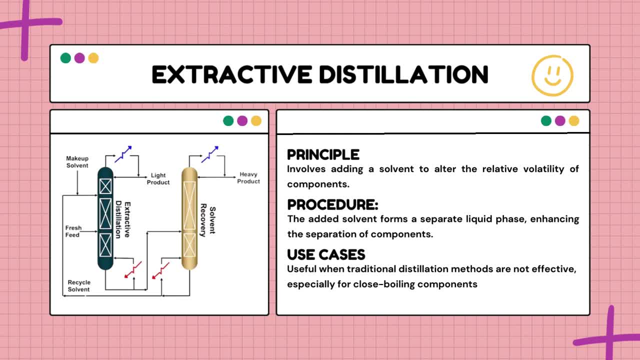 Extractive distillation is a separation method that also adds a solvent to change how components vaporize. This creates a separate liquid phase, improving the separation of the component, especially when they have separation. So let's look at the principle. Imagine extractive distillation as a strategy to make the components in a mixture play by. 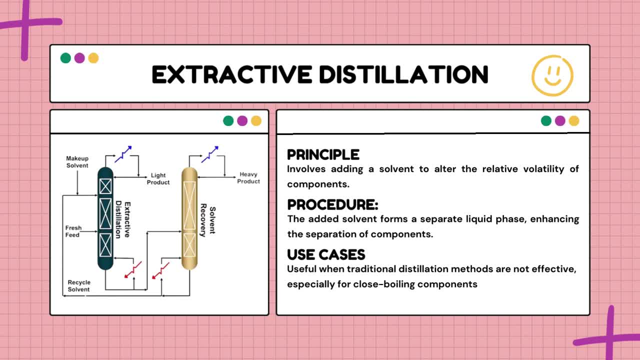 new rules By adding a solvent. it's like introducing a referee to the vaporization game, altering the willingness of the components to turn into a vapor In the procedure of extractive distillation. when close boiling point components make distillation tricky, a solvent is added. 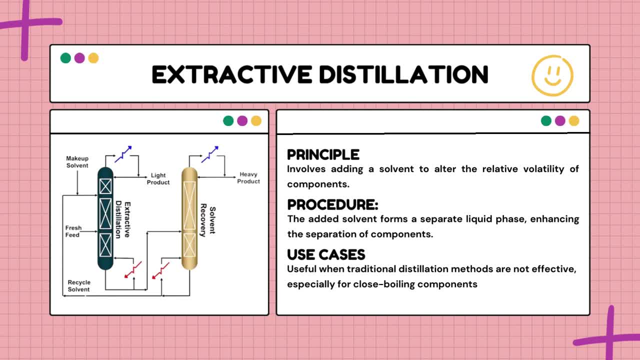 This solvent becomes a game changer, influencing how easily component transforms from the liquid to vapor. The added solvent don't just mix in. it forms a separate liquid phase. It's like creating a separate team in the game. This new phase enhances the separation of the components, especially those with similar 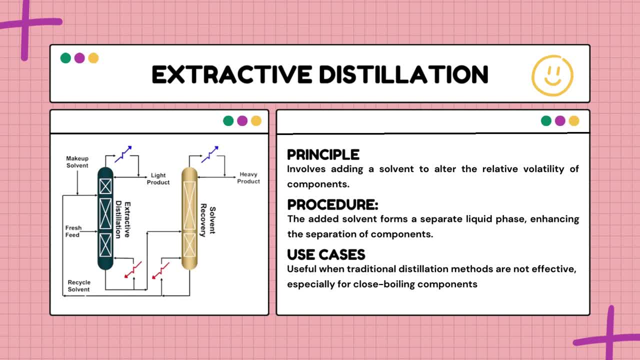 boiling points. With this solvent in the play, the components that might have behaved similarly due to the traditional distillation now have a different role. It's like giving each component a distinct jersey, making them easier to identify and separate. Okay, guys, so this was about the procedure or the working of extractive distillation. 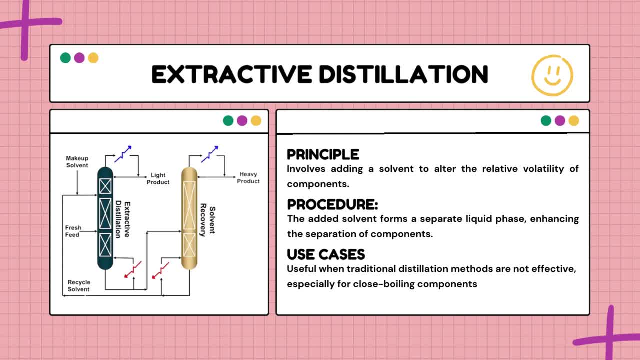 Now looking at the use cases. Extractive distillation steps up when the traditional method struggles with the components that are too cozy in their boiling preferences. When dealing with close boiling components, This method becomes tricky. This method becomes a valuable tool. Okay. 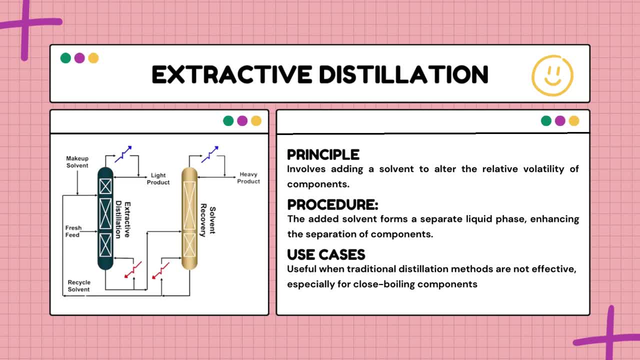 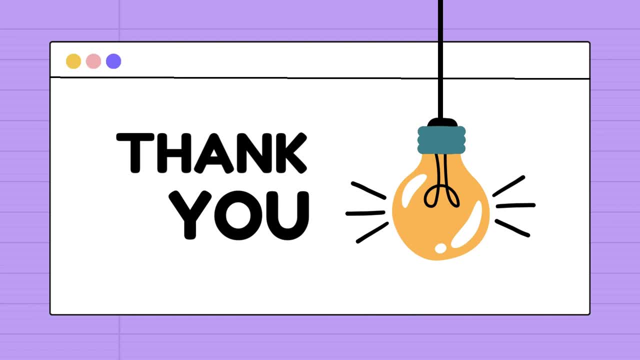 So, guys, this was about the extractive distillation And that's the end of this video where we discussed about various types of distillation. But particularly in this video, we talked about simple distillation, fractional distillation, steam distillation.